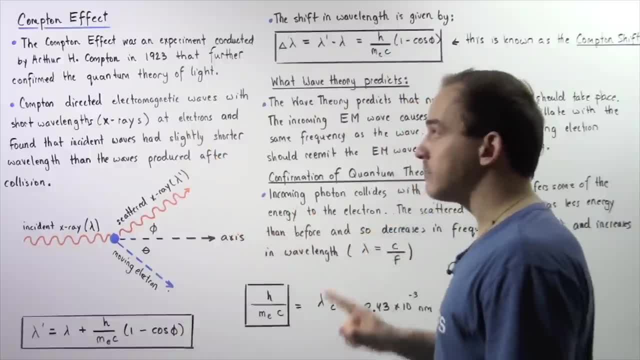 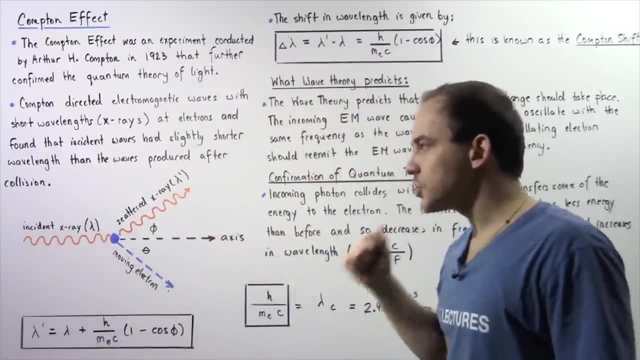 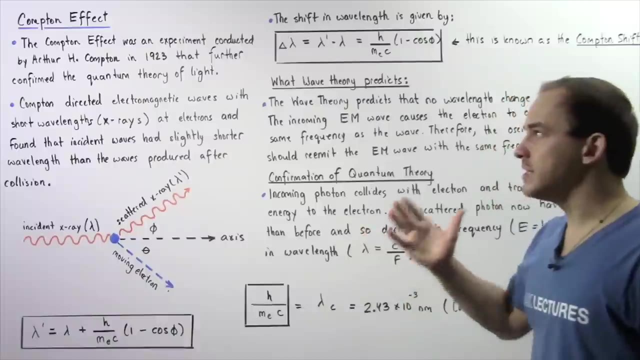 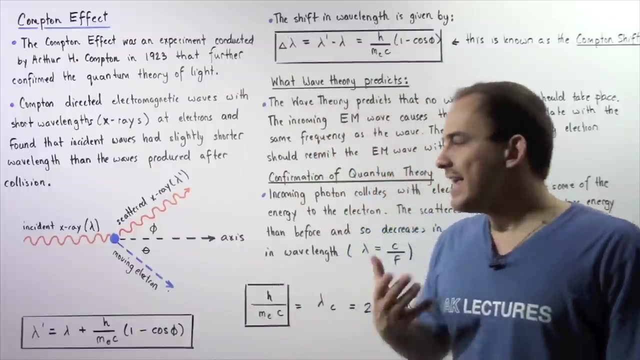 the horizontal axis, And what Arthur H Compton found was that the wavelength of the scattered X-ray was slightly larger than the wavelength of the incident X-ray, and this effect became known as the Compton effect. Now, using the conservation of momentum and the conservation of energy, he was able to 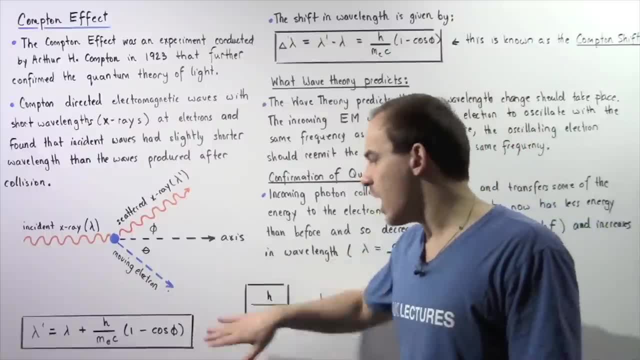 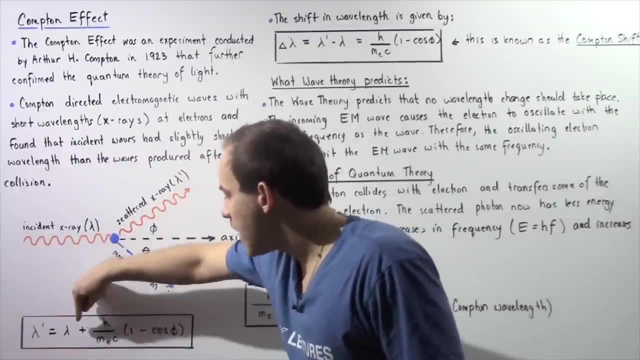 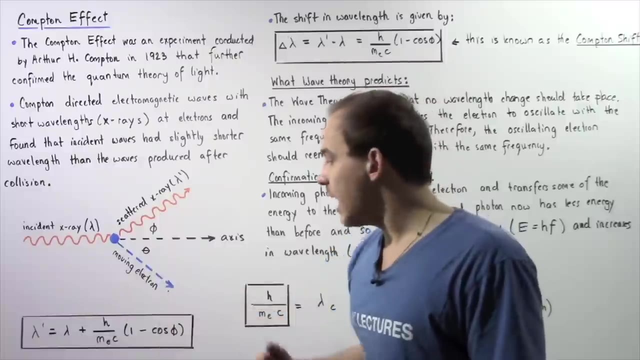 derive the following equation, which we're going to derive in a future lecture: So Our lambda prime is equal to lambda plus h divided by m, e, the mass of the electron multiplied by c- the speed of light, where h is Planck's constant- and this is multiplied by 1 minus. 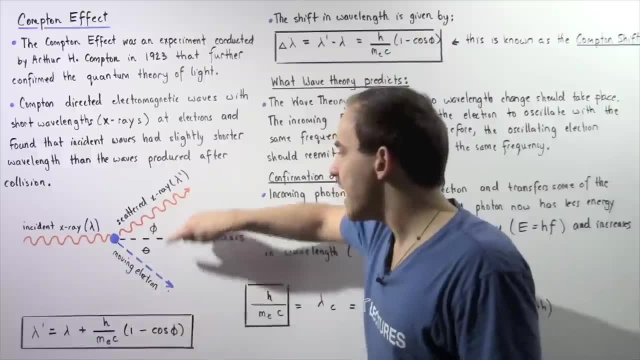 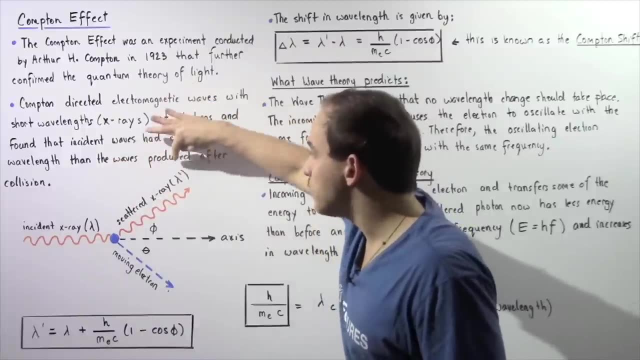 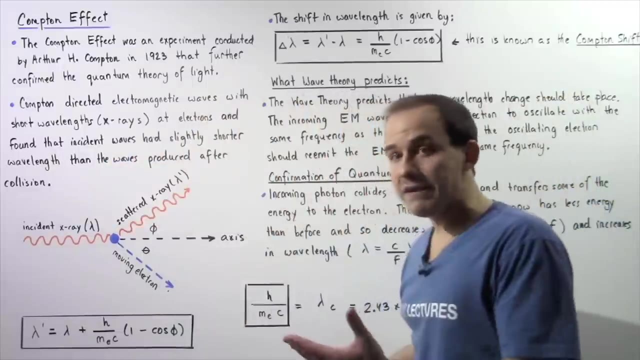 cosine of the angle phi. So once again, the angle phi is the angle between the horizontal axis and the scattered X-ray. Our lambda prime is the wavelength of the scattered X-ray, And this is the wavelength of the scattered X-ray. So We had an X-ray and our lambda is simply the wavelength of our incident X-ray. 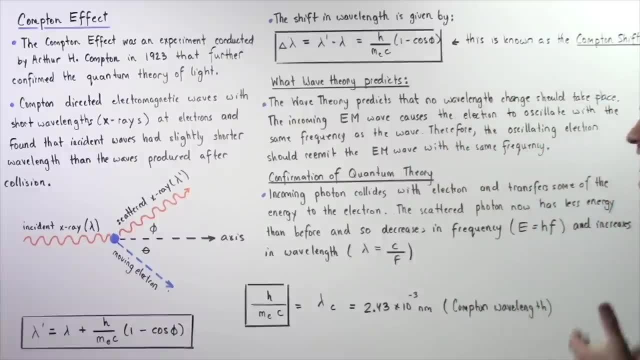 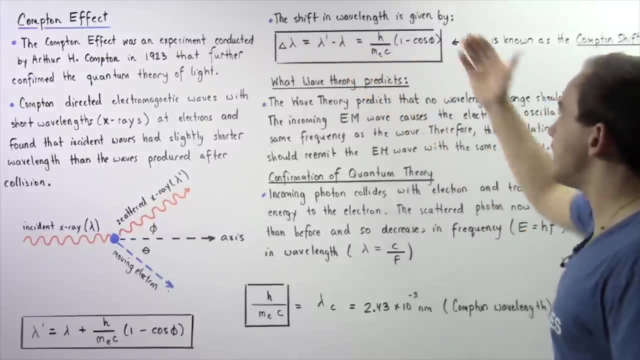 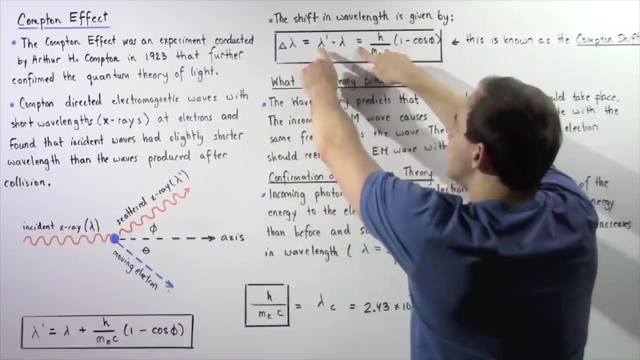 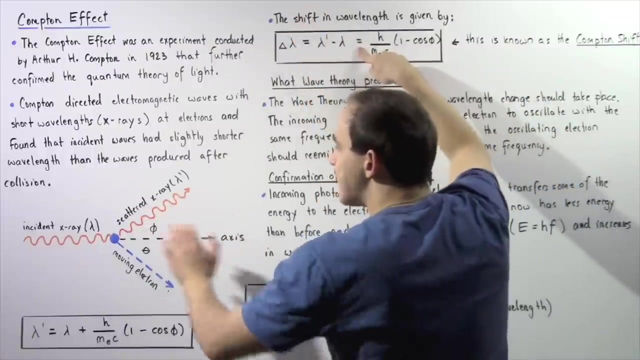 Now, using this equation, we can also determine a quantity that became known as the Compton shift. So the shift in wavelength is given by. well, the change in wavelength when this takes place is simply given by lambda prime minus lambda. So we place the lambda prime first, because that represents the larger wavelength quantity. 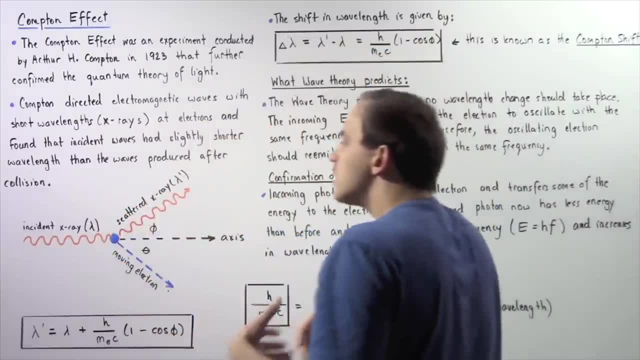 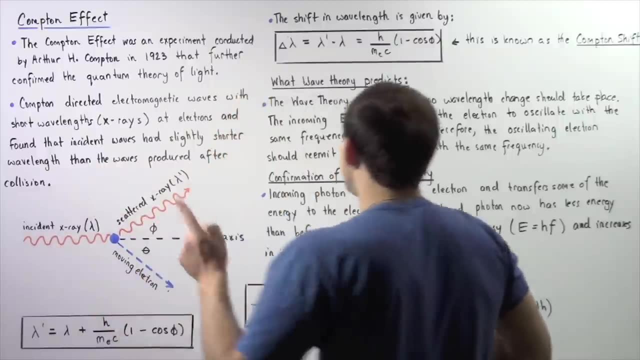 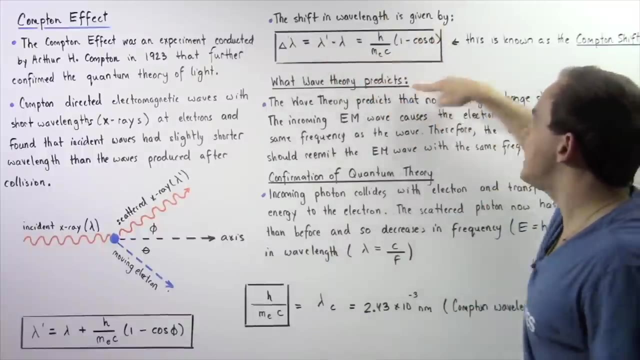 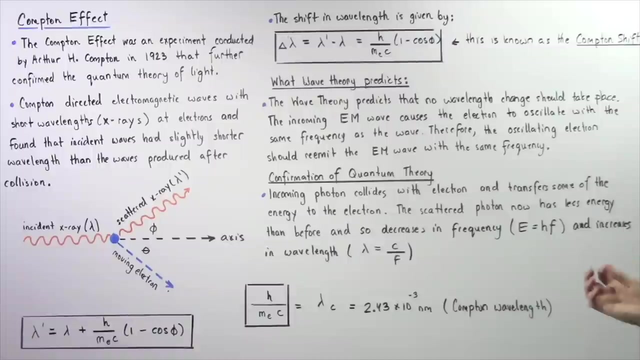 So, remember, when the collision actually takes place, the wavelength of the scattered X-ray is increased compared to the initial wavelength of the incident X-ray. So if we use this equation and subtract these two quantities, we get the following result: So This quantity became known as the Compton shift. 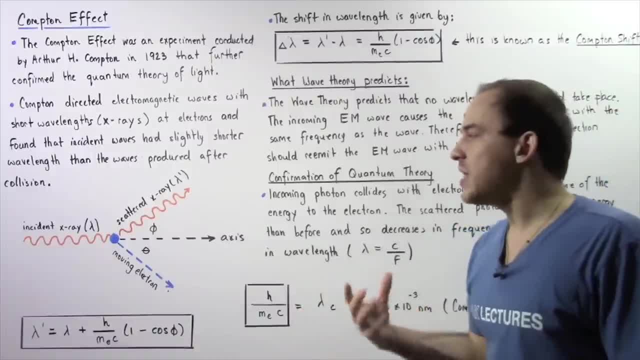 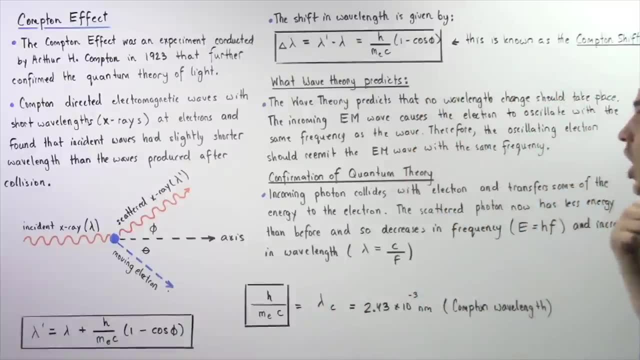 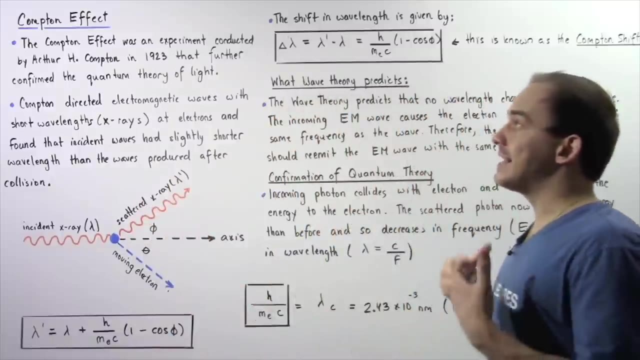 It represents the shift or change in wavelength that takes place when the X-ray, when the electromagnetic wave, hits this electron. So now the question is: how exactly did the Compton effect prove, or how did it essentially confirm, the quantum theory of life? So first let's examine what the wave theory of life is. 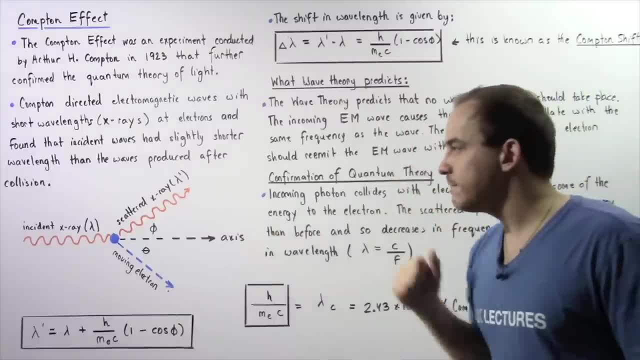 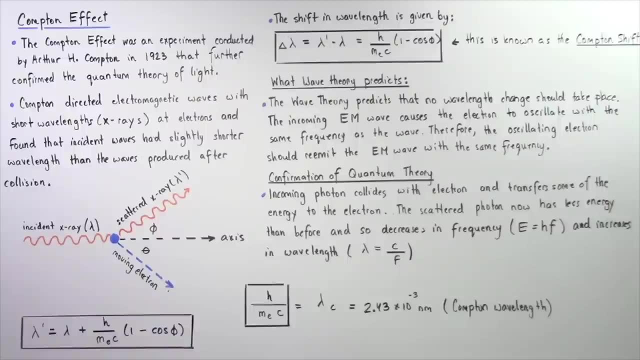 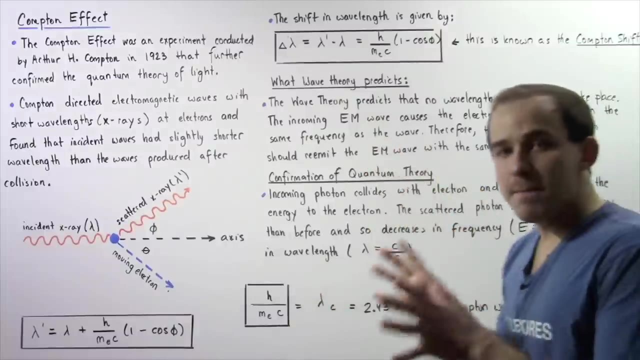 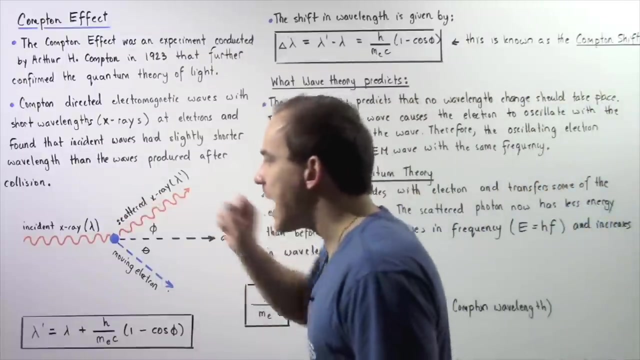 So The wave theory of life predicts the results to be for this particular experiment. So basically, the wave theory predicts that no wavelength should take place, And that's because the incoming electromagnetic wave basically causes our electron to oscillate at the same exact frequency as that particular electromagnetic wave. 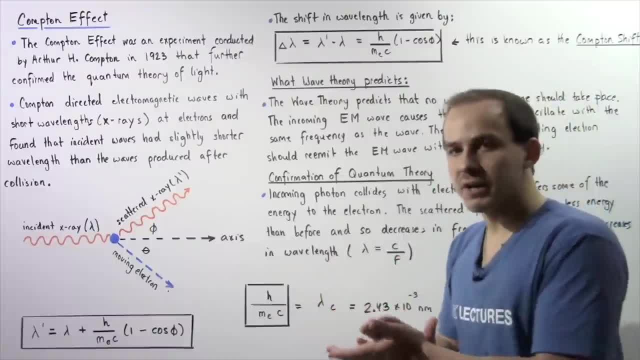 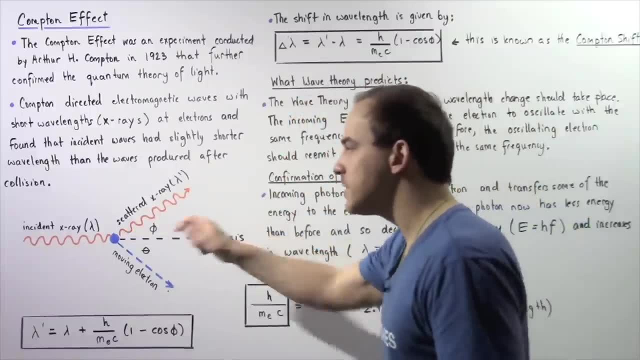 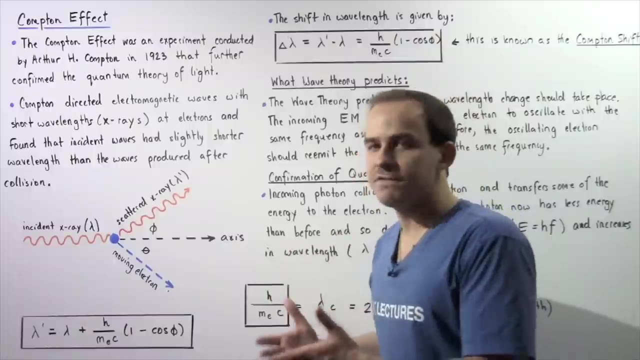 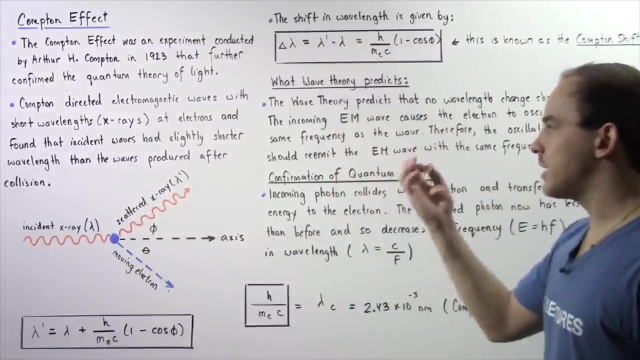 So when that electron re-emits That electromagnetic wave, The frequency of that scattered X-ray should be the same as the frequency of the electron. So that means there is no shift in frequency and that implies there is no shift in wavelength. Now, this is not what was actually seen when this experiment was conducted by Arthur H. 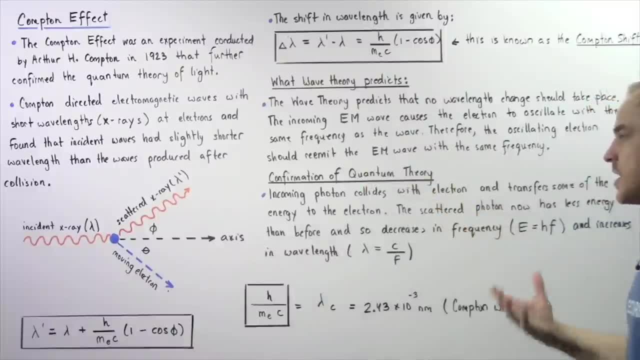 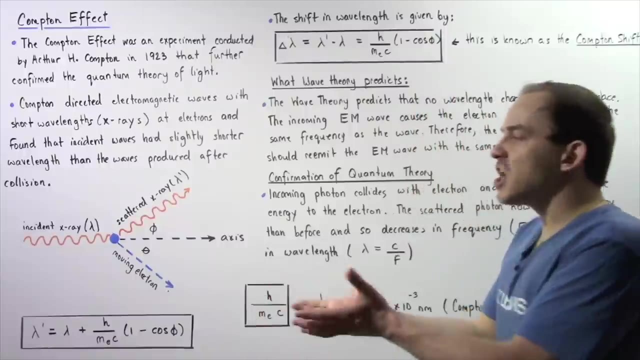 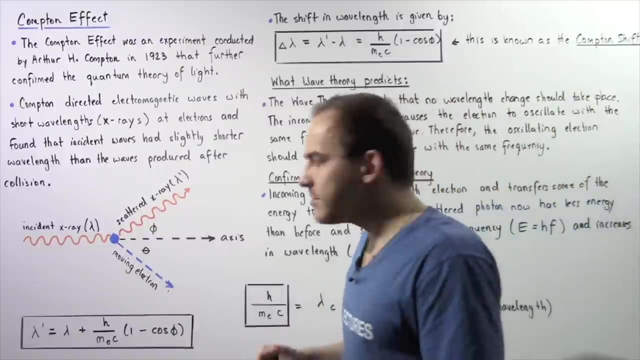 Compton And that basically confirmed the quantum theory of light, The fact that light consisted of photons. So Basically incoming photon collides with that stationary electron and that collision basically transfers some of that energy within the photons to that electron. So the electron gains kinetic energy and begins to move with some velocity. 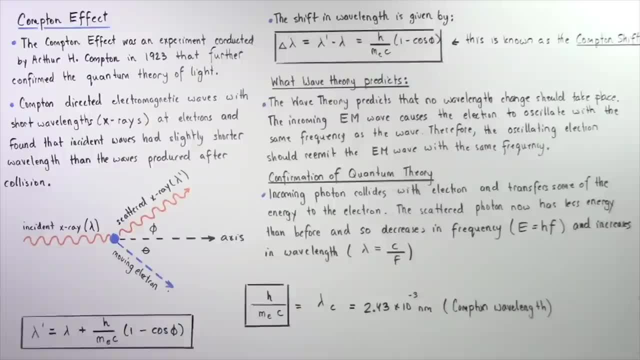 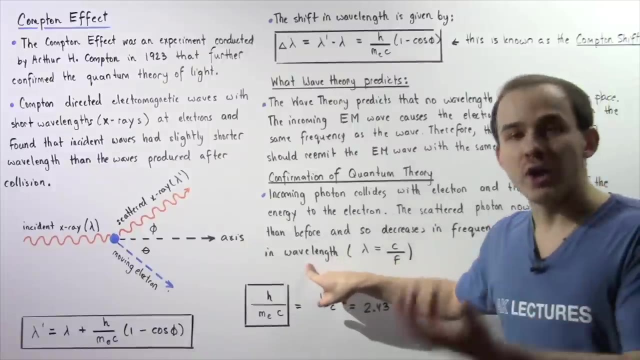 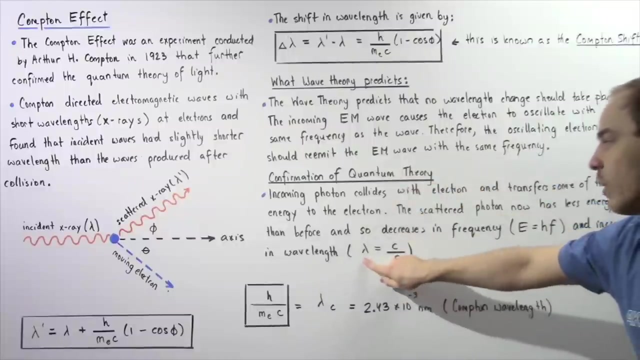 Now, the scattered photon now has less energy than before, And because it has less energy- And energy depends on the frequency- Less energy means a smaller frequency And a smaller frequency means a greater wavelength, As per the following formula. So if the frequency decreases, 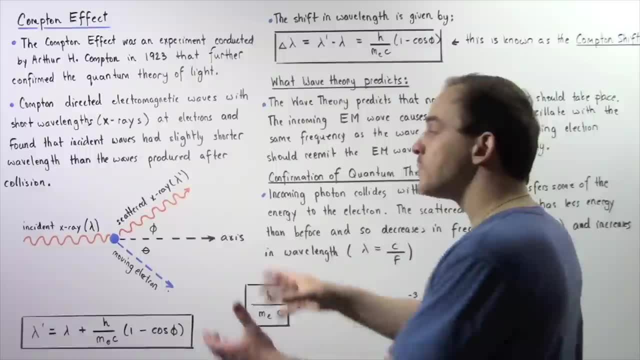 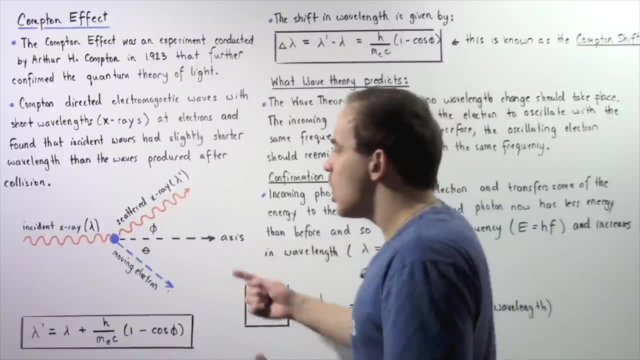 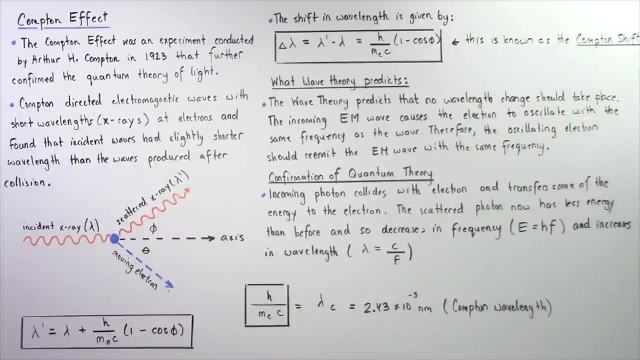 The wavelength will increase. And that's exactly why a change in wavelength takes place, Because some of that energy within the photons is transferred to the kinetic energy of that electron, And that is propelling that electron to move with some velocity. Now let's go back to this equation for just a moment. 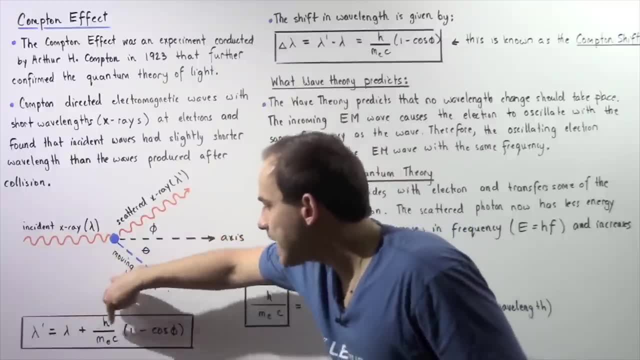 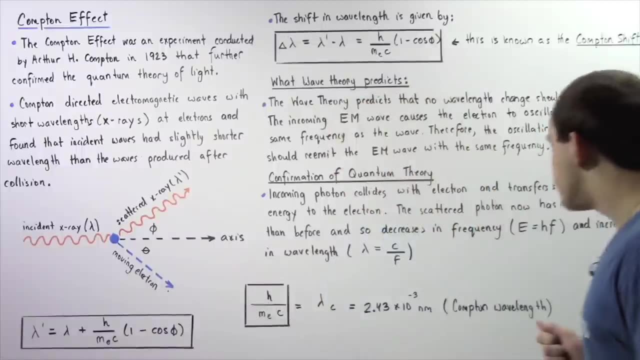 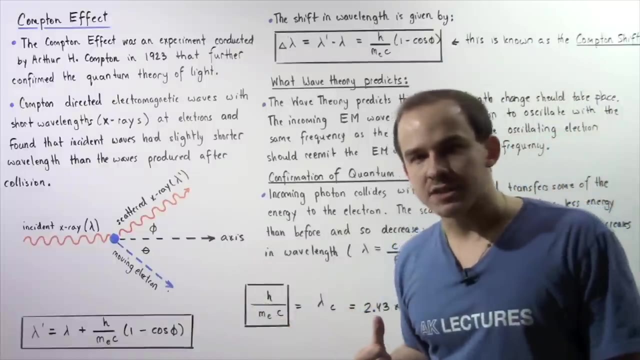 So let's examine the following ratio: H divided by M, E multiplied by C. So this ratio has a specific name And it's known as the Compton wavelength. That is given by lambda C, where C stands for Compton. So basically it's the wavelength of